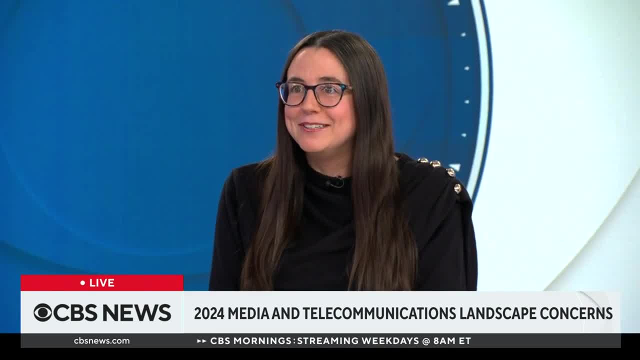 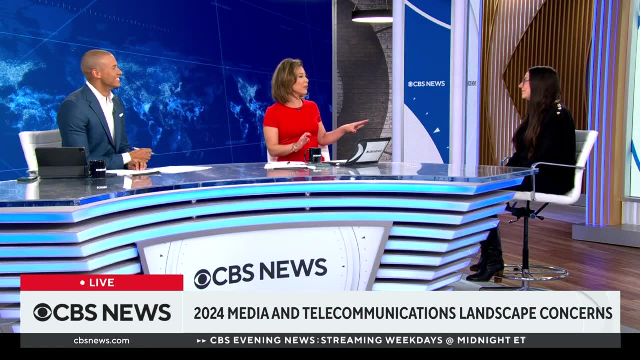 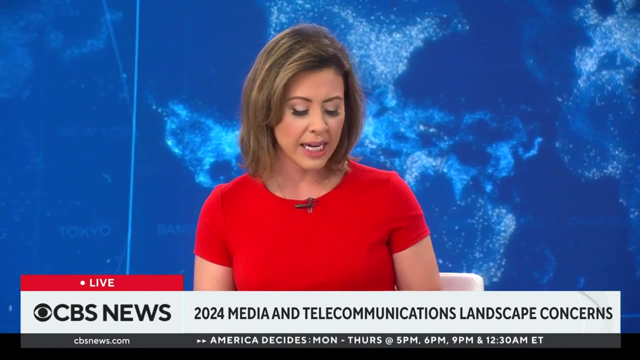 So really going into next year, something's going to happen with Paramount. Ooh Errol's starting us off strong. you know asking for a friend, But whenever we're looking at an upcoming election year, there's a lot of investment, particularly in television, news and ad sales. 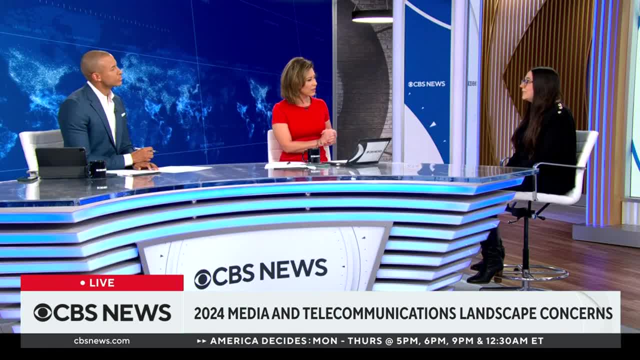 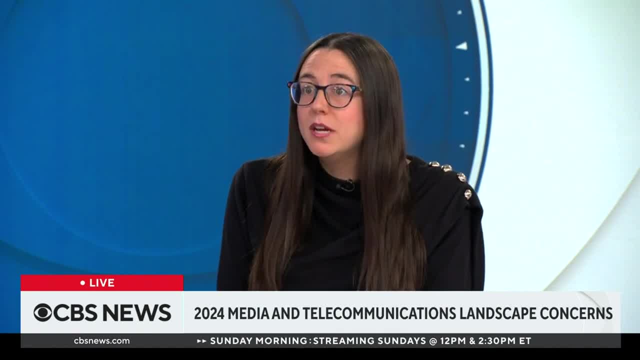 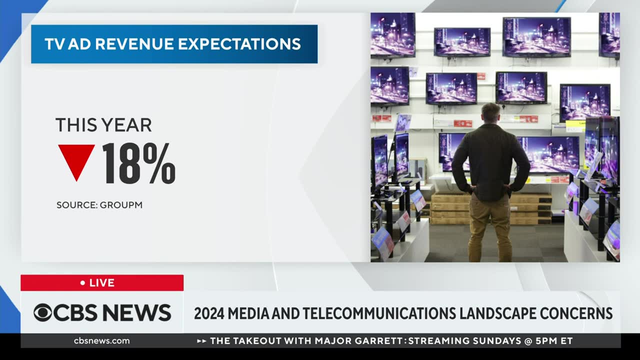 The hope is that it will get a little bit better, though, with the election. The issue is, though: there's so many platforms to spend advertising money on these days. right, I was just covering billboard companies. There's hope that there will be more political windfall of ad dollars to billboards, right. 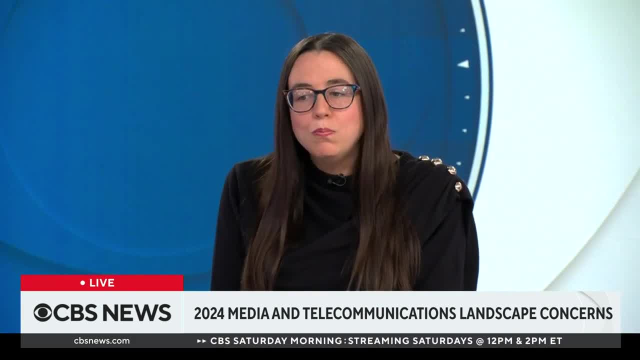 It's not just television that's fighting for those dollars. So overall we'll see a bump, but it's not probably as big as we're used to And you know, I think it's going to be a big deal. 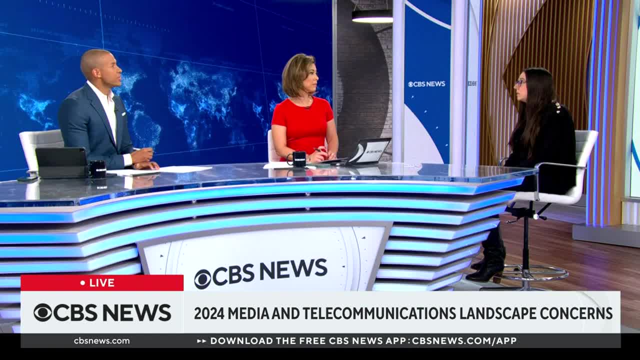 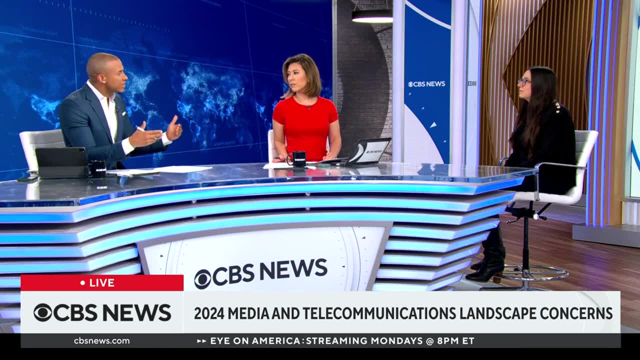 And not big for those companies that we just mentioned. We should also mention that it's Warner Brothers, Discovery, NBCUniversal. All media companies are kind of showing interest in purchasing something. Inflation is cooling, though The Fed's expected to reduce rates next year. 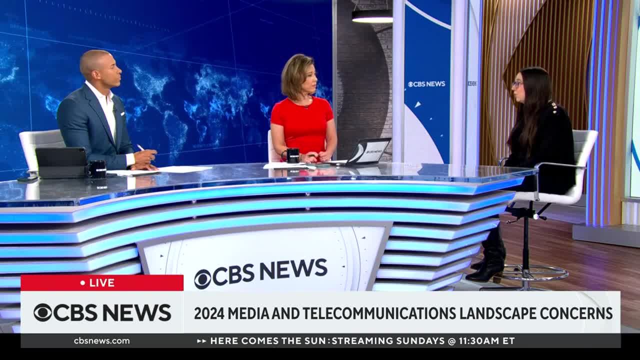 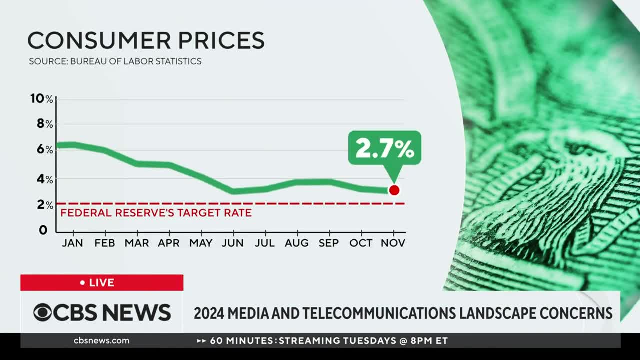 Might that play a role. I think that will 100% play a huge role. A reason for, as a media deals reporter, it was a quiet year- I was not as busy as I wanted to be, And I think one of the main reasons was exactly what you said. 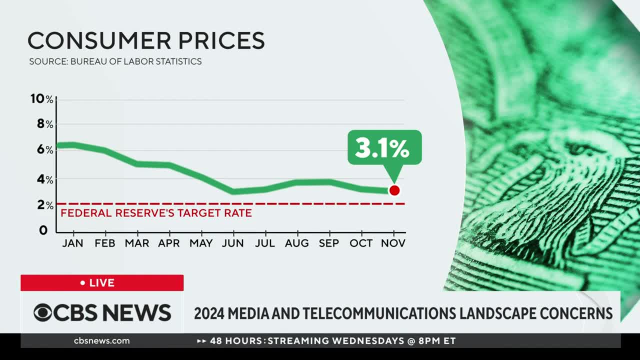 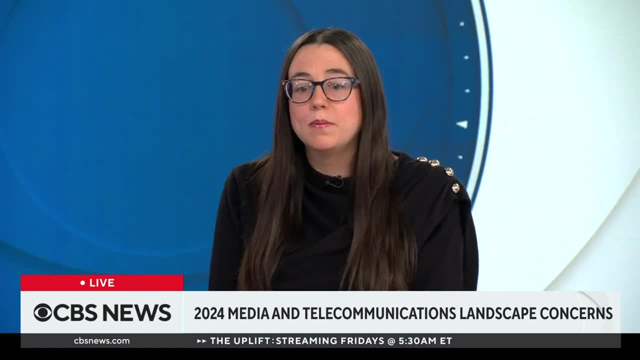 That's what people told me The interest rates were. There's less cheap money that way. You're not in really buyers and sellers are not interested in doing deals in that market. So we didn't see as much. We just heard from the Fed that they're planning to lower the interest rates, right? 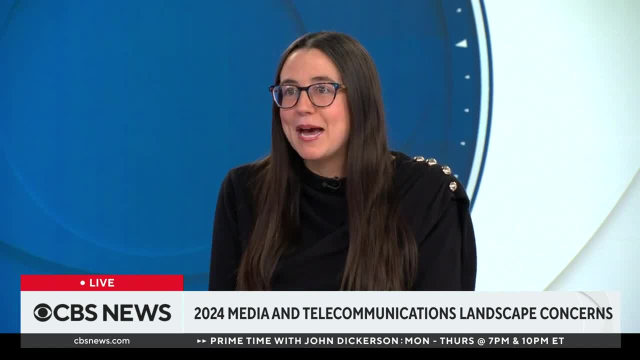 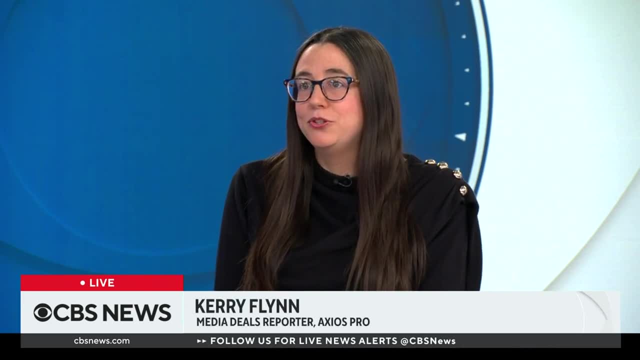 So that is gung-ho, deals a-blazin'. Let's see what happens now. There's also the thought of regulatory concerns. That was something that was really plaguing this past year. I mentioned Paramount's sale of Simon & Schuster. 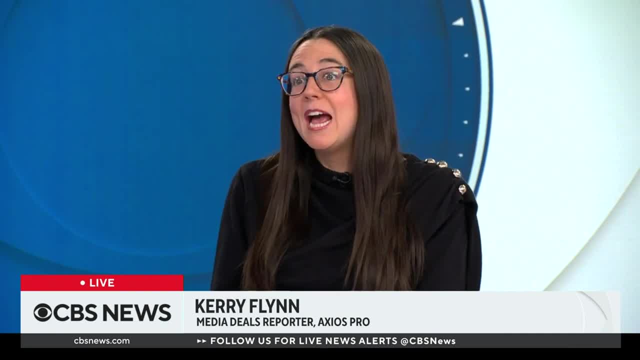 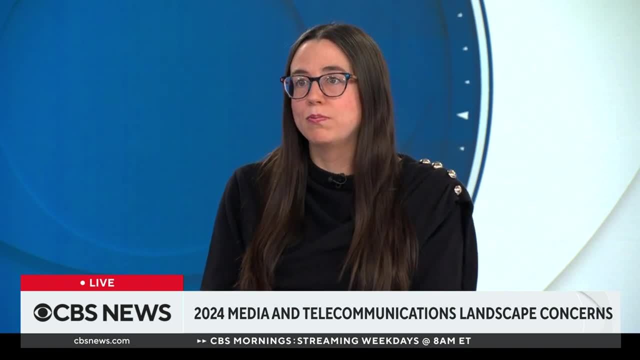 They were supposed to sell that to Penguin Random House, another book publisher, And that deal got blocked by a federal judge over antitrust concerns. So there was a pause there. but we also have seen deals go through, The latest example being Microsoft buying Activision Blizzard. 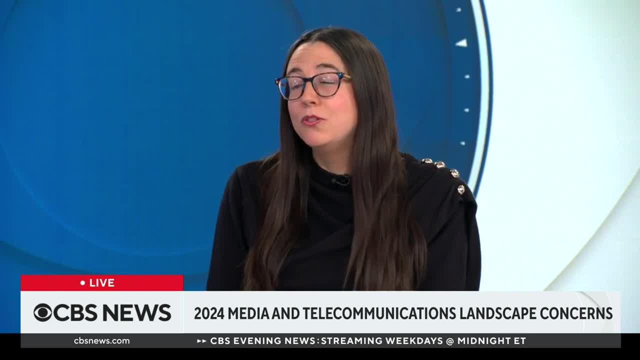 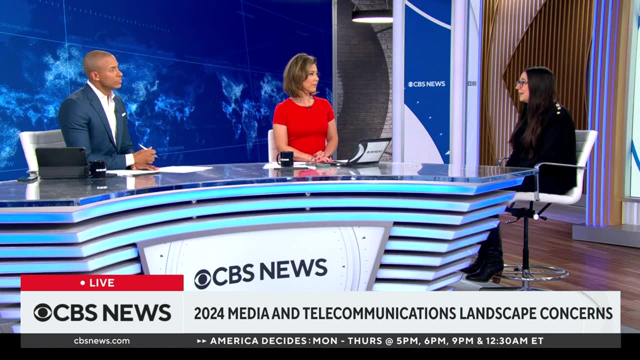 So, even though there was really a lot of tension over that this past year, the hope is going forward. it'll get better. But again back to politics. we're going to have to see who's in office and whether you know that will decide who has the power there.